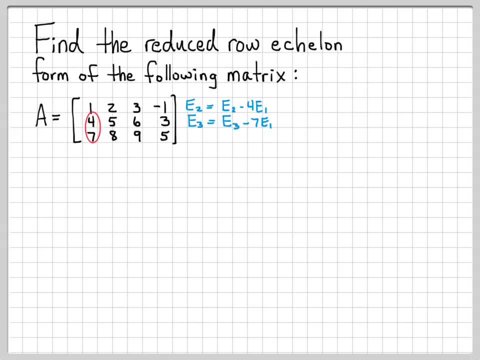 itself minus seven times equation one to cancel out these four and seven right there. So equation one stays the same. I end up with a zero there for equation two And negative three here, because five minus two times four is a negative three. And if you just continue the simple. 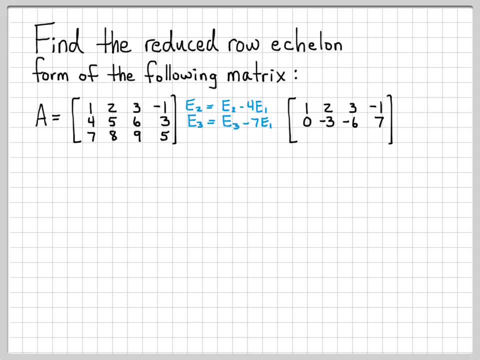 computations there you end up with a negative six and a seven. And then I'll do similar type operation here for the third row. The third row minus seven times the first row gives me a zero there, because seven minus two times four is a negative three. And then 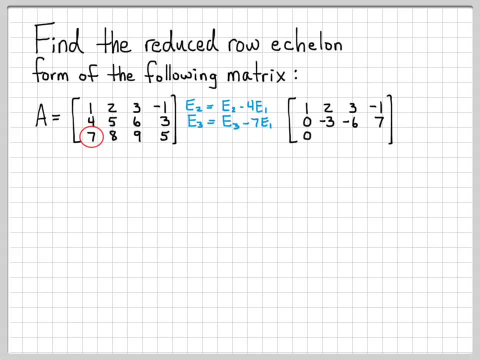 I end up with: seven minus seven times one is zero. And then I end up with: eight minus 14 is a negative six. Nine minus 21 is a negative 12.. And five minus a negative one times seven ends up being five plus seven, which is 12.. So I'm off to a good start. I have a one right. 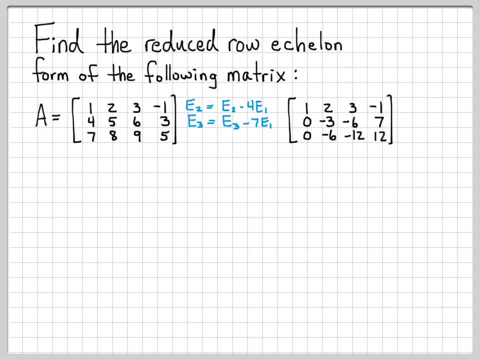 here and I have zeros below it. But now in the second row, the first non zero thing that I come across is negative three. So I don't like that negative three there, Same thing here. I don't like this negative six here either. So we're going to start working on this next column. So, if I let equation 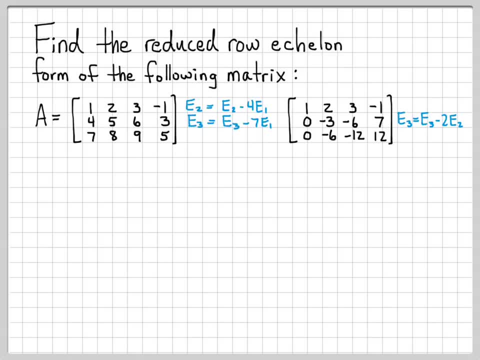 three equal equation three minus two times equation two. I can get a zero right there. So equation one and equation two remain unchanged. I keep a zero there, And then I'll have a negative six minus a negative three times two, which gives me a zero and a negative. 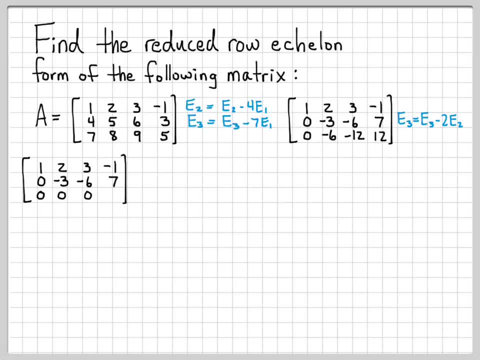 12 minus a negative two times a negative three. So I'm off to a good start And then I end up with a negative six gives me zero there as well, And then I get a negative two here. when I do 12 minus seven times two, it's 12 minus 14 is a negative two. Okay, so we're 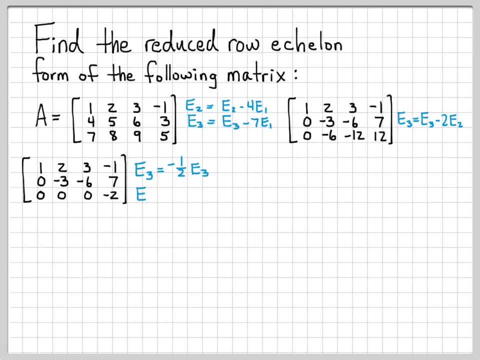 getting there. Got some zeros there. Let's go ahead and let equation three equal one half times our negative one half times equation three. we're going to turn this into a one because, remember, in any row, the first thing that I come across has to be a one. So, as 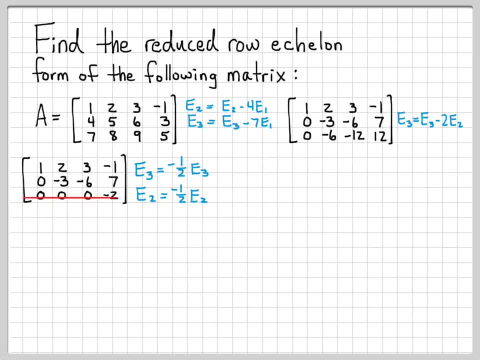 I'm going across this row. I have zero, zero, zero. then I have a negative two. I can't hit a negative two, I have to hit a one. So I can turn a negative two into a one by multiplying by negative one half, And then we'll do something similar here for equation. 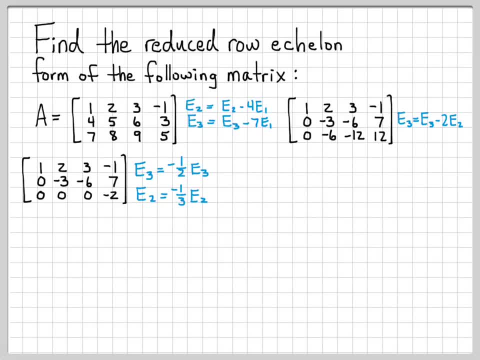 two. If we multiply, multiply equation two by a negative one third, that will turn a negative three into a negative one. we'll have that one sitting there like we'd like. So after we do this multiplication we have the one there. in equation two we get the. 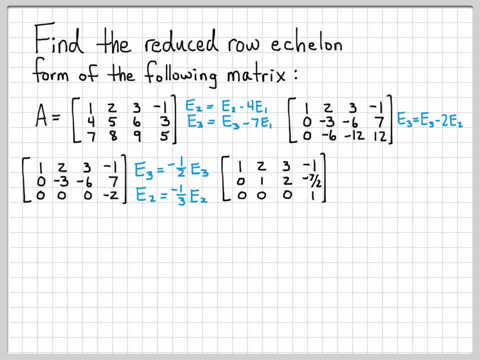 one in equation three, like we would like an hour. now we're getting there. we're almost, almost done. I have one with zeros below it. I have a one with zeros below it. The next thing that I need to do is get rid of some of these other entries right here. I let equation one equal. 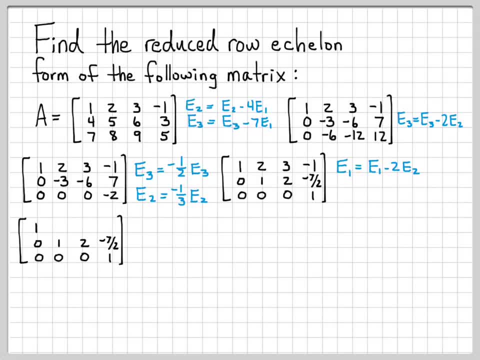 equation one minus two e two. So only equation one is going to change, only copy down e two and e three by themselves, without changing an equation one. I end up with a zero And with this then we'll go ahead and let equation two equal. equation two plus seven halves equation three. 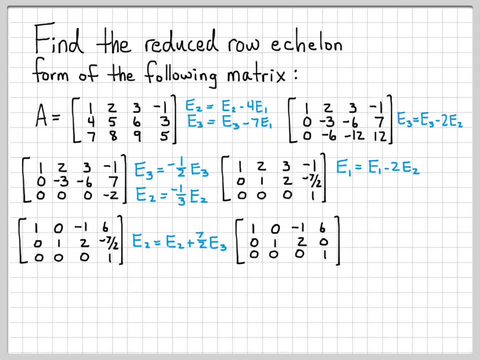 So I'm only going to change equation two: still have a zero there, still have a one there, And I can cancel out that negative seven halves. So after doing this I end up with this matrix right here. You might be wondering why are 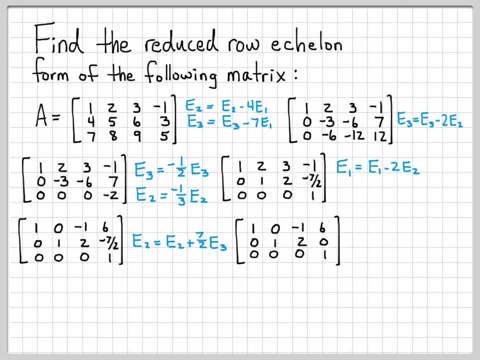 we trying to get rid of these entries. Well, one of the other rules about the reduced row echelon form is that any column that has a pivot- and these are what we call pivots, these ones that can be the only nonzero term there. So we're glad that we have a one right here. 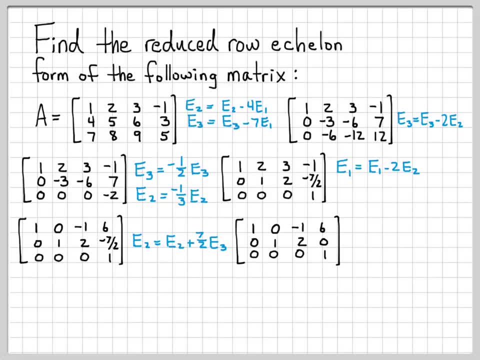 But the fact that these are nonzero is a problem, So we need to get rid of those. So I've gotten rid of one of those right there. I can keep going. if I let e one equal e one minus 63, we can get rid of this right here, And then we'll end up with this final matrix after. 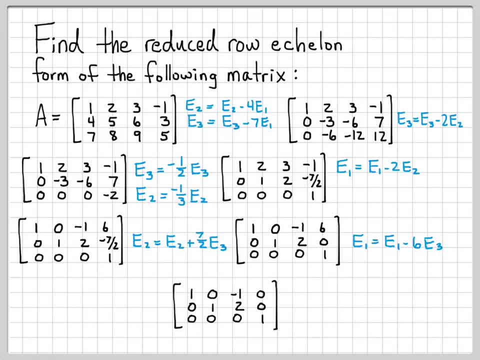 we do the computations, that looks like this: And this is, in fact, the reduced row echelon form of the matrix. I can check this And I can say: Hey, you know, let's get rid of this. the matrix. I can check this. 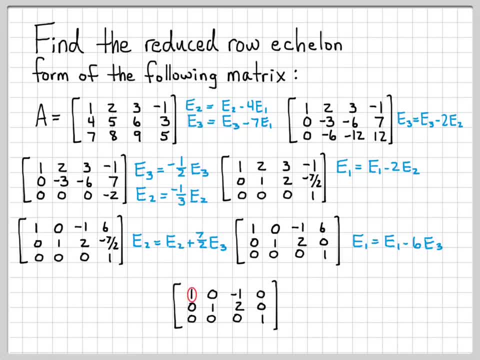 In the first row, the first non-zero entry that I come across is a 1,, and it is the only non-zero entry in this column. In the second row, the first non-zero entry that I come across is a 1,, and it, too, is the.